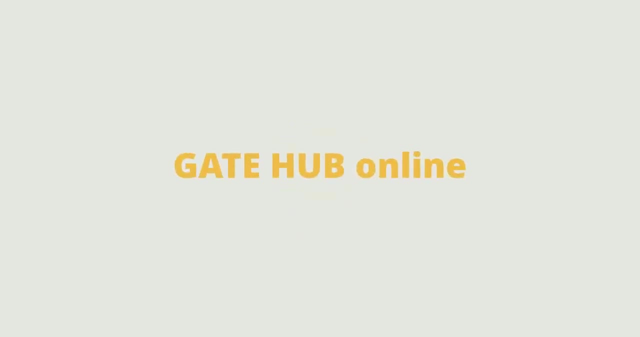 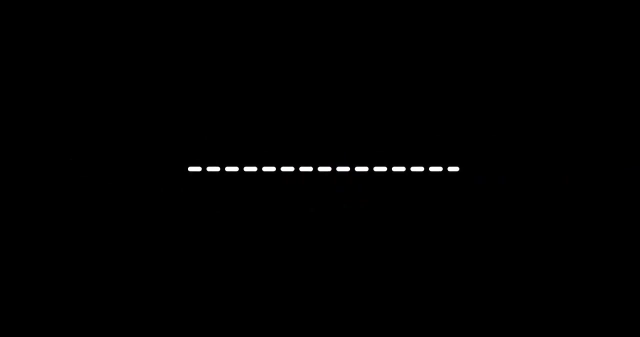 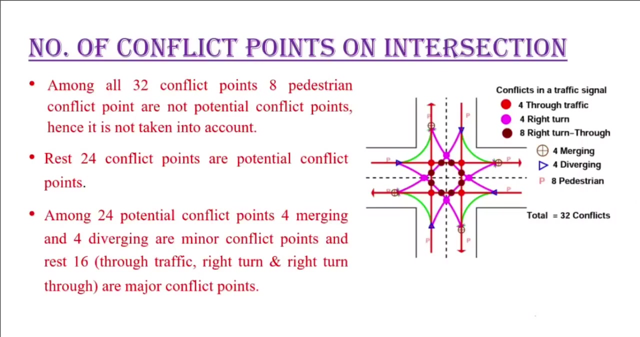 Hello everyone, Welcome to GitHub online. In this video we are going to discuss about number of conflict points on an intersection of a highway. Okay, before we discuss about the important points regarding the conflict point, let us know about the conflicts point. 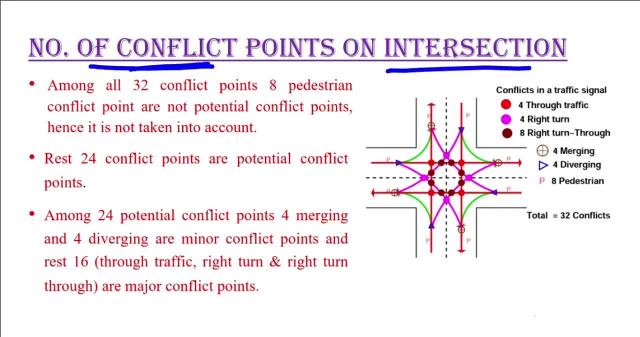 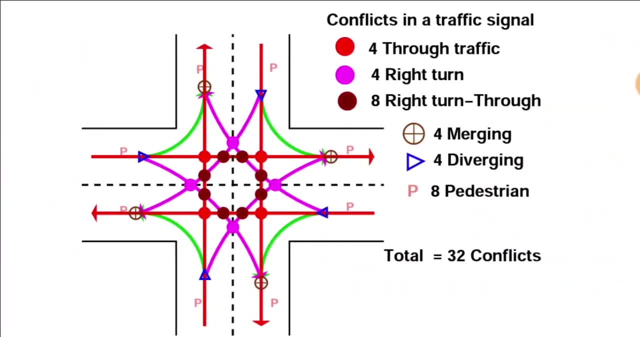 and how it can be find on an intersection. Okay, so, with the help of this diagram, we will understand what is conflict point and where it occur on a national highway. So let's see this figure by zooming in. Okay, see, here there is a two-directional traffic. 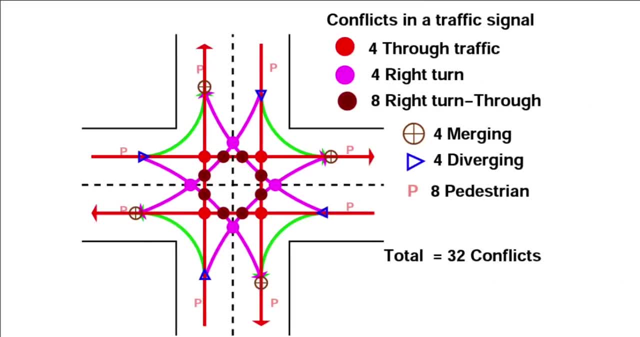 road, Two-way traffic is intersecting. There is an intersection. Okay. from here, our traffic movement is in the west and east direction and in the north and south direction. Okay, so see, both the roads are meeting at a junction and both of them have two-way traffic, Okay. 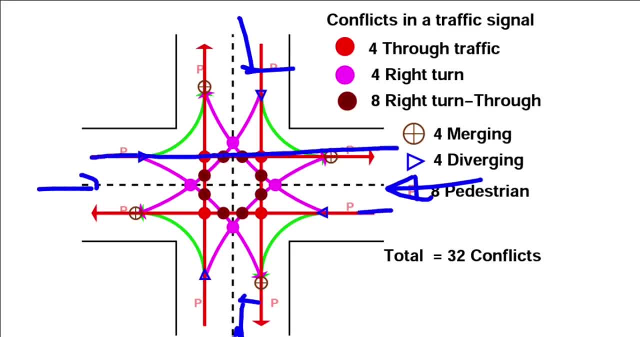 means if any traffic will move from here in this direction, from here in this direction, similarly, if it will move in this direction, then in this direction and in this direction. Okay, So this is the movement of traffic. Okay, so what is the number of conflict points? 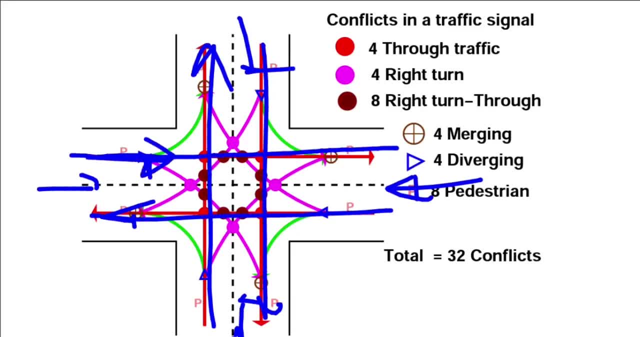 If our traffic movement is from here and there are three more directions apart from this here. here see, there is a movement from here apart from this, this is a three-direction. Okay, so when there is a movement of traffic from both the different directions, okay. 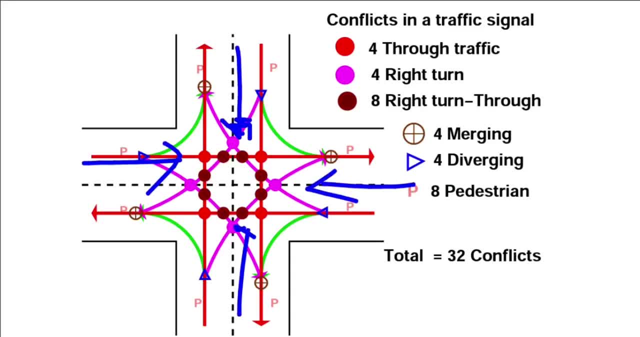 then at which point of both the traffic can be collision. So the number of points that will be collision, Number of Dana electric don't house fixed points, which means at that point of the system what we'll call both points is number of conflict. right means at that point we'll have省. 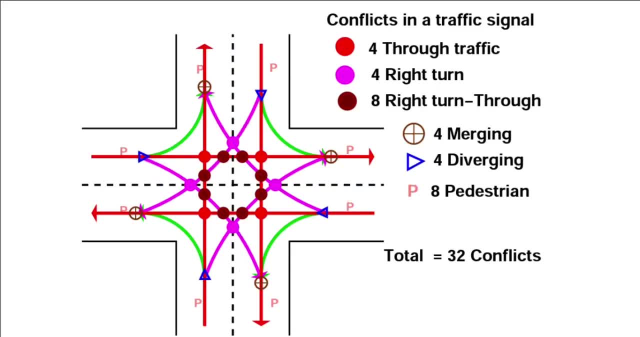 chances Look like this. Here we'll Define how to find it Right First, if we look in the east and west direction, then we take the way traffic movement can be seen. there will be traffic like this and from here, Suppose that if this moment goes from here left to right, so where will the traffic come НА? 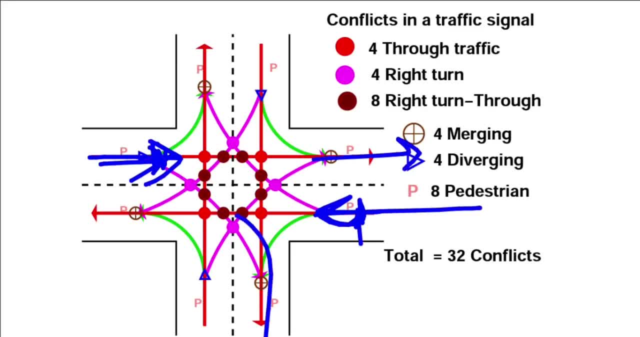 toDoes the update. Look here, there we're going. Alright, let's decide, Observe Where. Whether it goes from here to, it will go to here, Okay, so you will make sure Or move here or here in three directions. 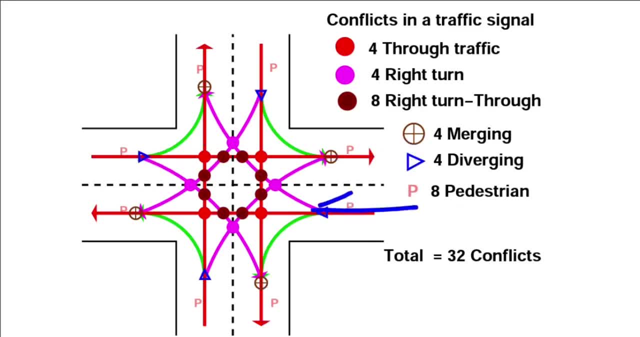 Okay, Clear. Similarly, if it comes from east to west, one can go straight here in the west direction, One can move in the north direction here and one can move in the south direction here. Similarly, if it's coming from the north direction, then what is that? 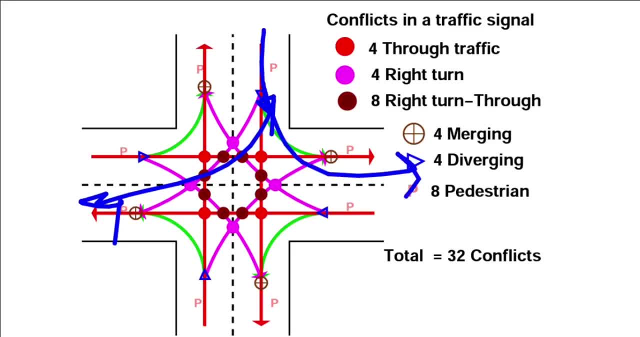 One can go in the west direction here, in the east direction and in the south direction. Similarly, if it moves from the south, it can move in three directions. Is it clear? So look from here. I am telling you clearly here. 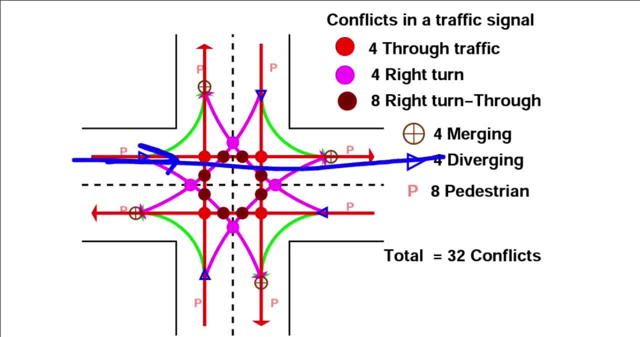 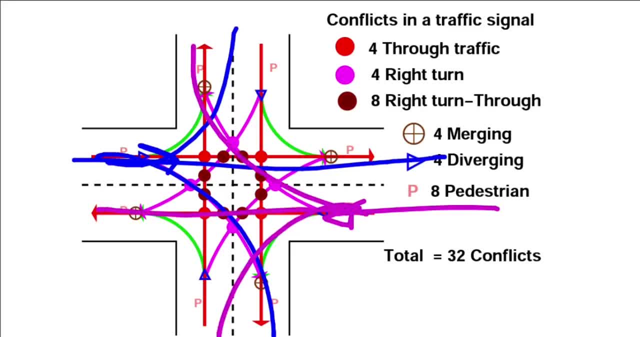 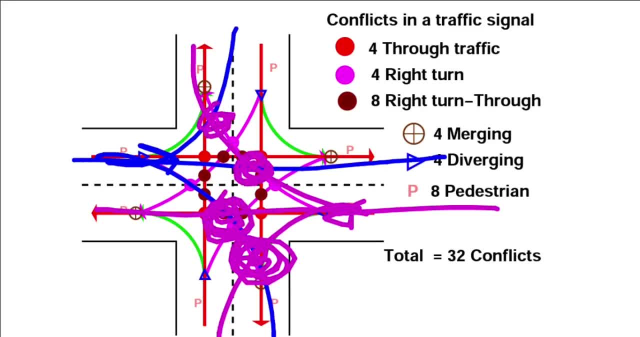 One at this point, Is it clear? Then, from here, you are getting four points. Is it clear? Four points are getting When, in this type of four directions, our traffic movement will be Means: One direction, Two directions, Three directions. 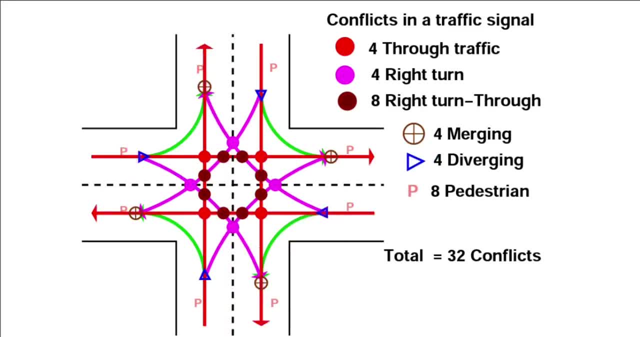 And Four directions. If there will be movement in such four directions, Then total number of conflict points we will get How much? Thirty two, Is it clear? See which one from this? The one that is showing here in red color. 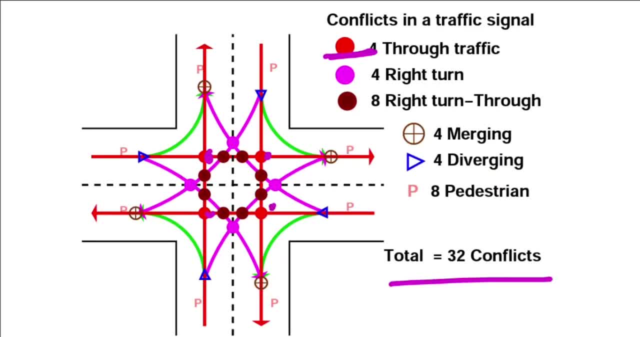 Means At this point, This one, This one, This one, Is it clear? So these four, What will we call it? Through traffic conflict point, And the one that is showing here in pink color. Means Here, Here. 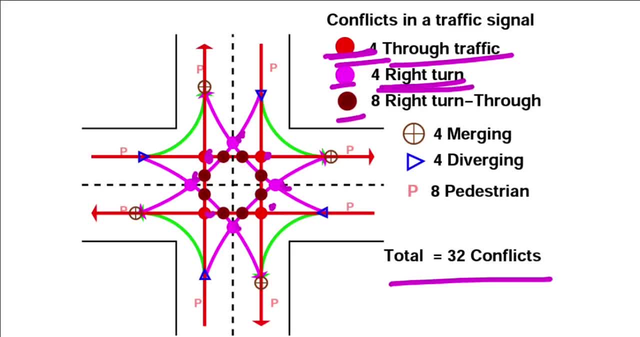 Here Here. What is this Right turn conflict point Means Here, Here, Here, Here Here Here Means Total eight. How much is this? This is right turn through conflict point. Is it clear? And 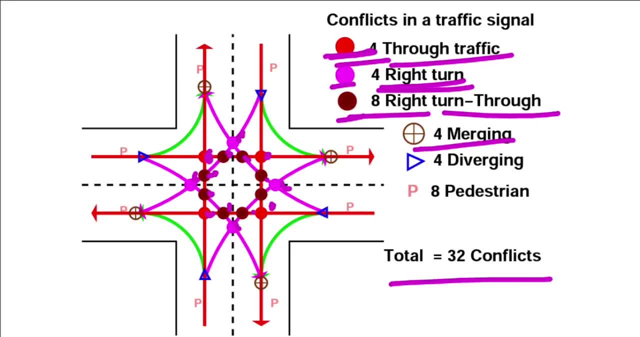 Four, We have merging conflict point. See Where plus point is happening Here. two traffic is merging. One is this And one is this. Is it clear? Similarly, Here is looking like an arrow. What is this Diverging conflict point? 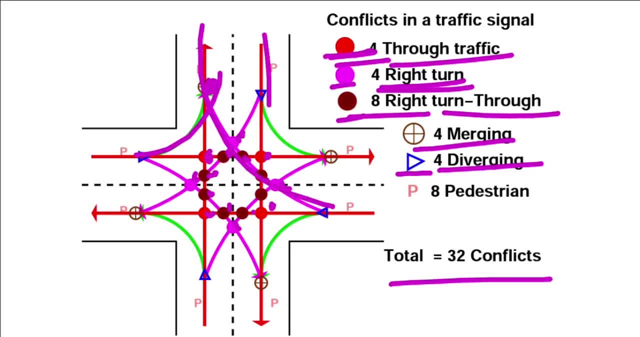 Is it clear? Means: See, From here traffic is coming. Where is this going And Coming from here? Here. So Both are diverging here. So What is this Diverging conflict point? This is also four. 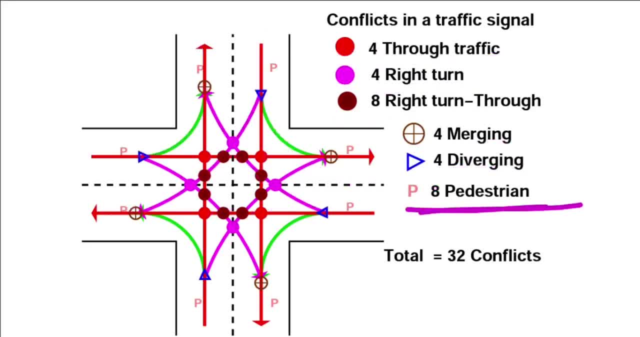 Is it clear? Similarly, Eight: We have pedestrian Where P is happening Here, Here, Here, Here, Here And Here Is it clear? So We have eight pedestrian conflict point. Is it clear When we will do the sum of all this? 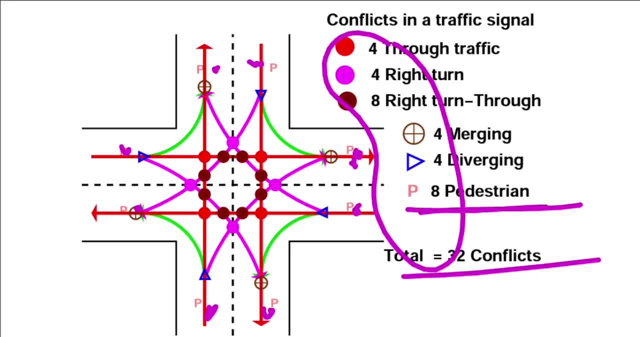 Then What will be our total number? Conflict point Means Total thirty two points. What is our accident? Or We can say Collision of two traffic. Is it clear? What do we call this? Conflict Number of conflicts point. 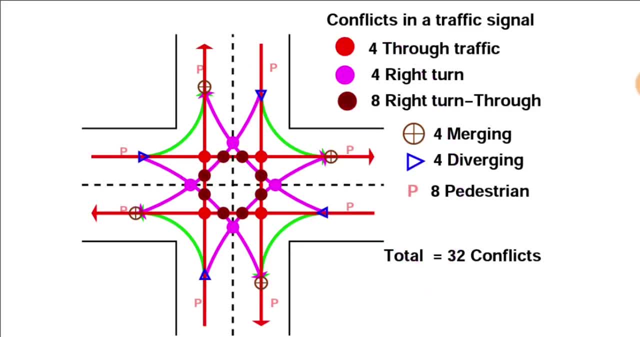 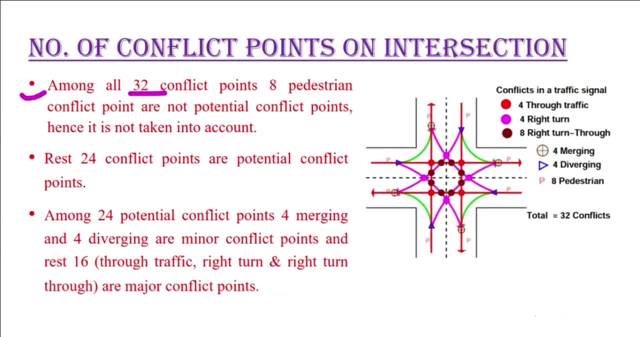 Ok, So Let's see. Regarding this, Some important points, Is it clear? So See, What is this? Among all thirty two conflict points, Eight pedestrian conflict points are not potential conflict points. Hence It is not taken into account. 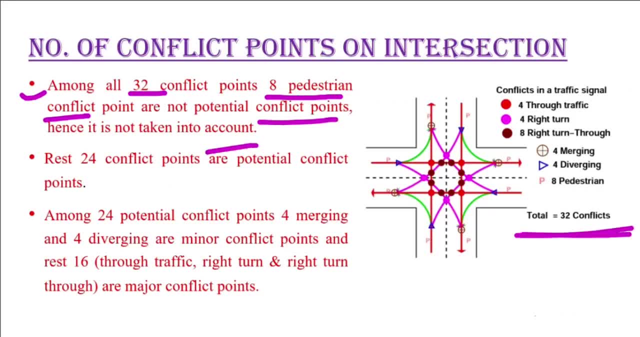 What is this, This total number of thirty two conflict points, Out of that, Eight pedestrian conflict points. Is it clear? What is that? There is no chance of accident in that. Hence, What is that? There is no potential conflict point. 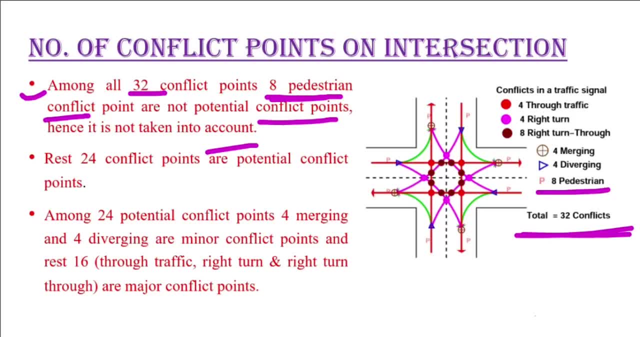 And We cannot consider this. Is it clear? So When Thirty two minus eight, We will have Potential conflict points. How much will it be? Twenty four Means Rest. Twenty four conflict points Are potential conflict points. 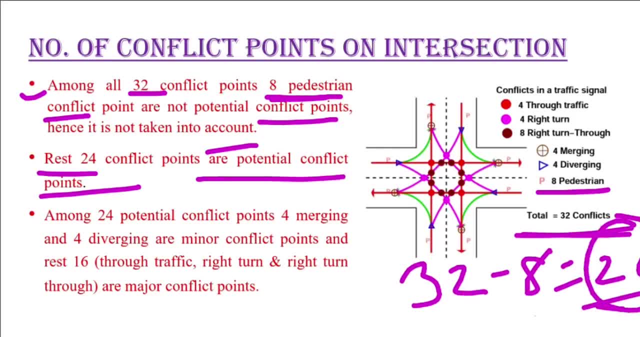 Is it clear Means When we design Intersection In that We design Twenty four number of conflict points. Is it clear? Now, See From this Twenty four, We have Potential conflict points. Is it clear In this? 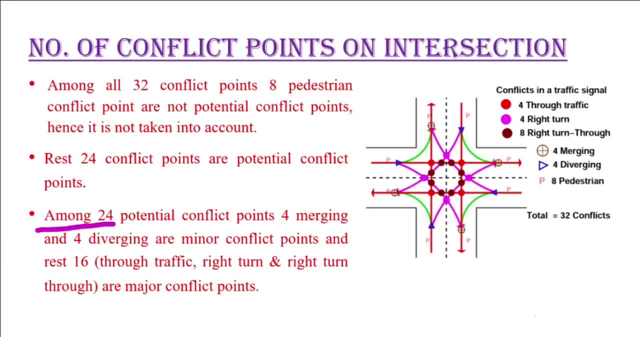 Twenty four conflict points. What happens Among Twenty four conflict points? Four merging And Four diverging Conflict points Are Minor conflict points And Rest sixteen, Sixteen, That is Through traffic Right turn And